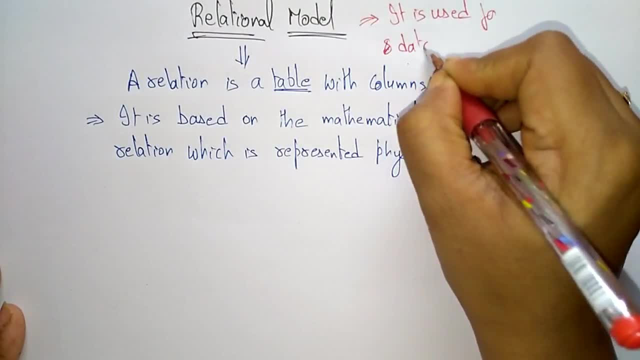 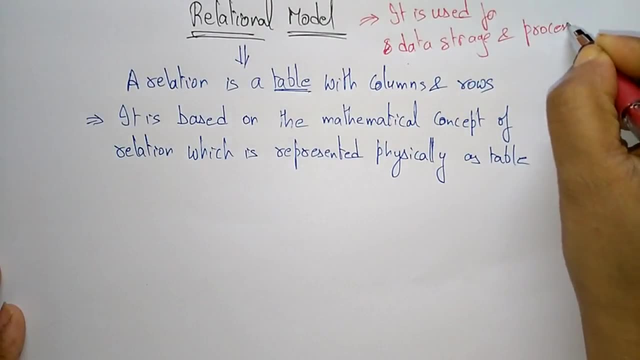 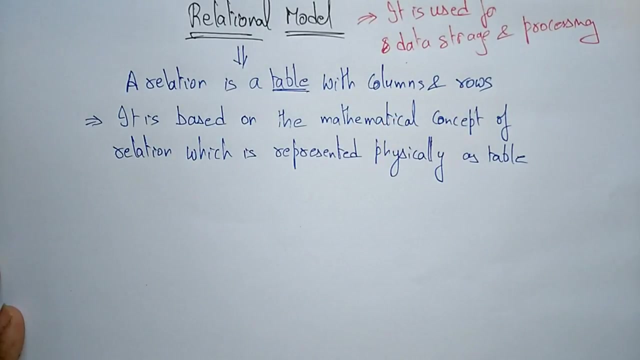 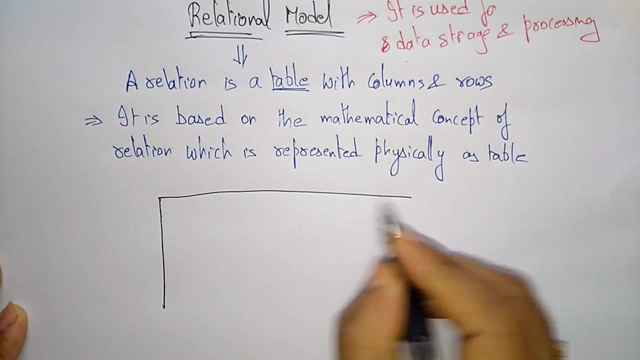 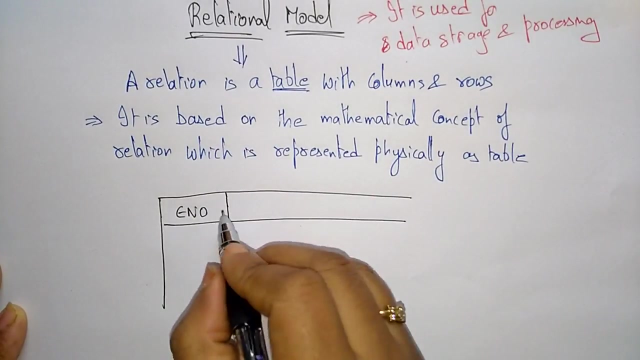 For data storage and processing. So the main use of the tables, that is, the relational model, is for storing the data and as well as the processing. So let us take one table. So this table consists of the fields, So the fields is also called as attributes. So employee name, employee number, employee name address. 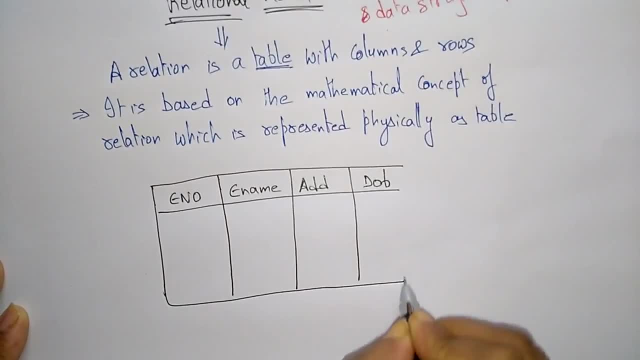 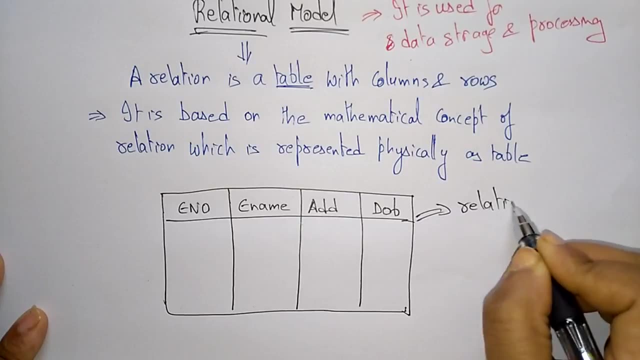 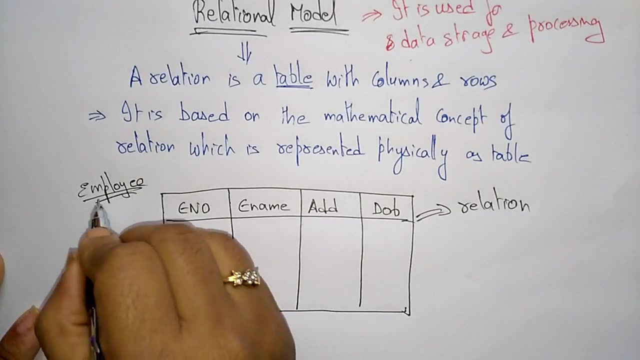 Date of birth. So this is a table Means it is a relation, So the table name is: employee. Employee is a table name So that you call it as a relational name. So another name for this is: table name is a relation name. 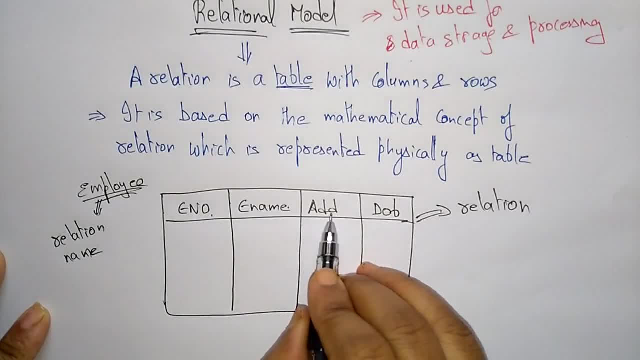 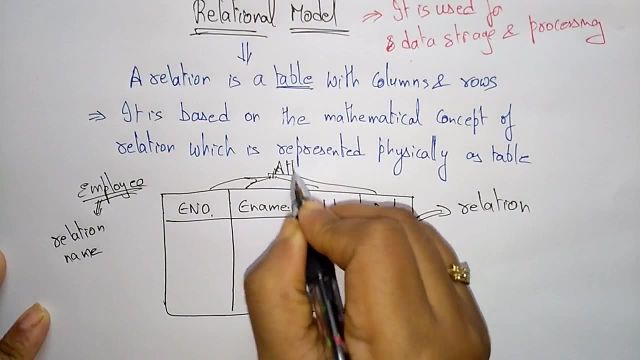 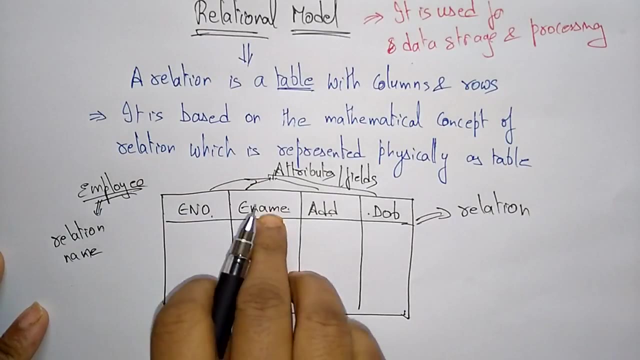 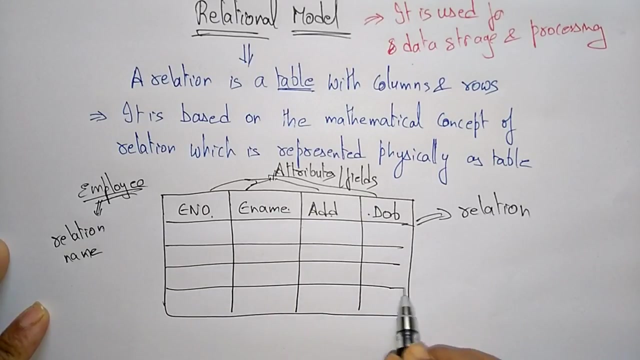 And whereas employee number, employee name, address, Date of birth, All are called as attributes, So these are attributes. or you call it as a fields. So these column names, you call it as a fields. And coming to each row, Each row, you call it as a tuples. 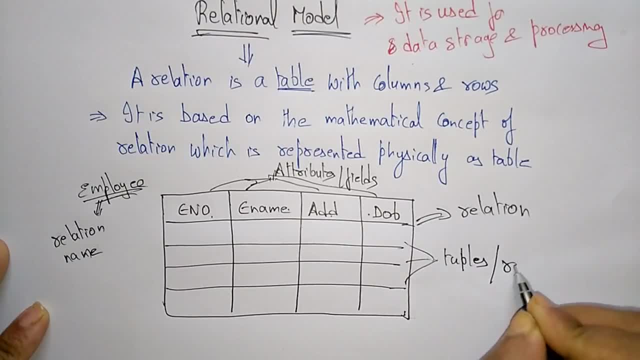 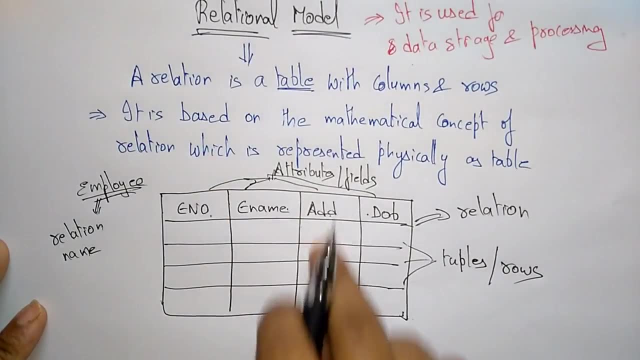 Tuples or rows. So the rows Rows, you call it as a tuples, Whereas the columns you call it as a attributes. So these are the terms that you have to be remember while you are discussing or creating the tables: Attributes, you call it as a columns. 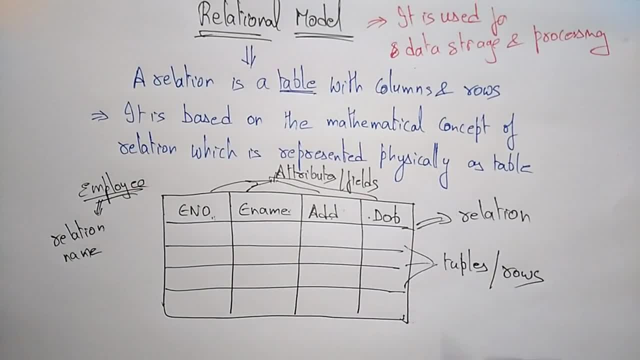 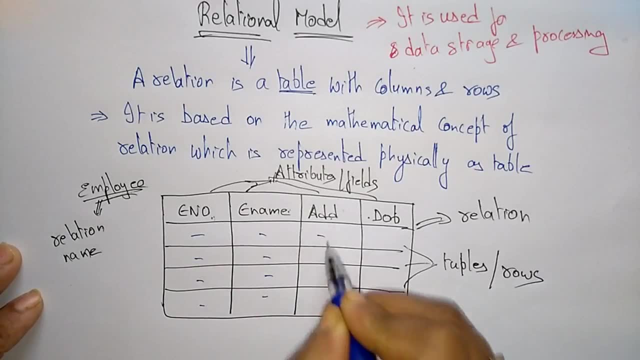 And the rows. you call it as a tuples, So actually the values that are present in each columns, or the rows, So those you call it as a domain: values, Domains. So these are the terms that you have to be noted. Attributes: 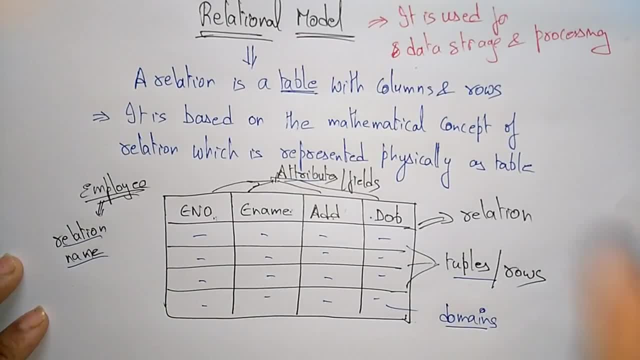 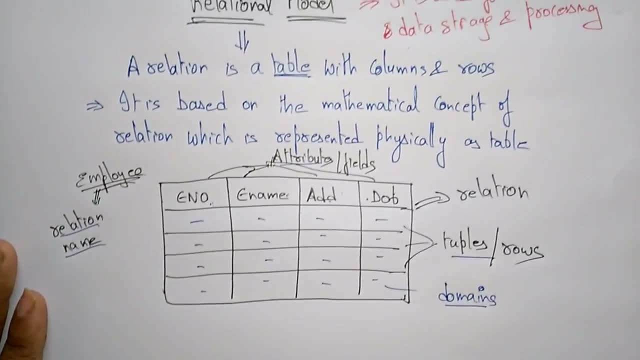 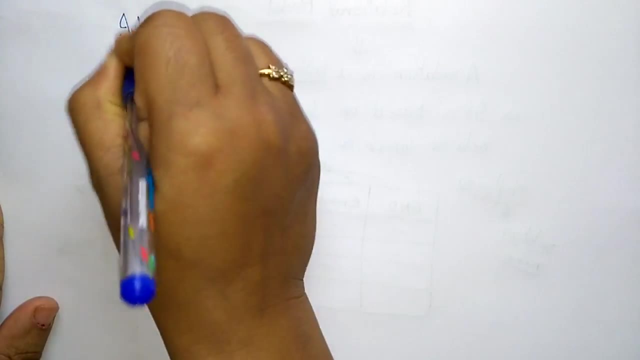 Tuples Domains Relational name. So these are the terms that are occurred in the while you are creating the tables. So let me write the informal and the formal terms That came across in the table. Informal terms And the formal terms. 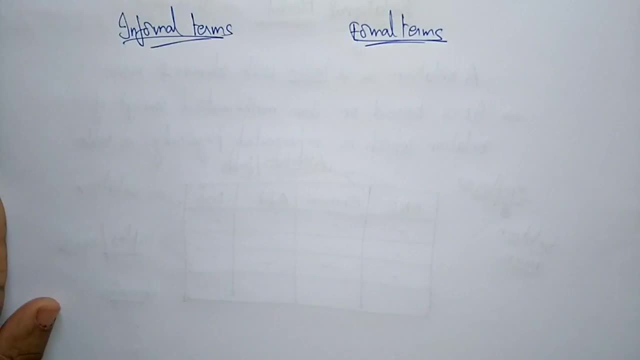 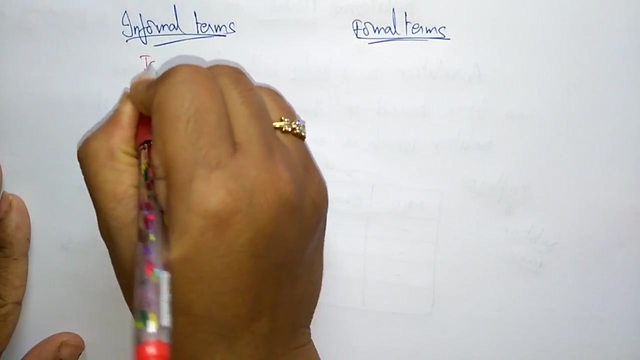 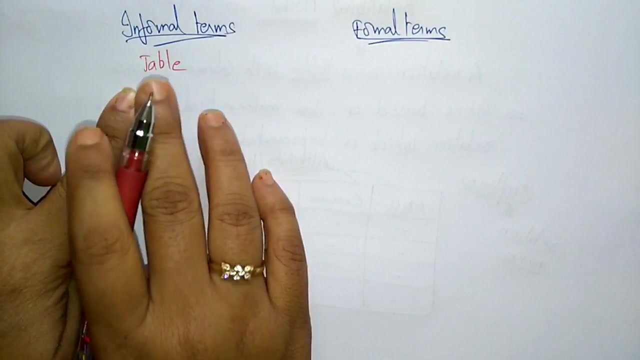 So in the relational model concept you will get across some formal terms. So informally you call it as a table, So the informal name for the relational model is the table. So formally you call it as a relation, So the another name for the table. 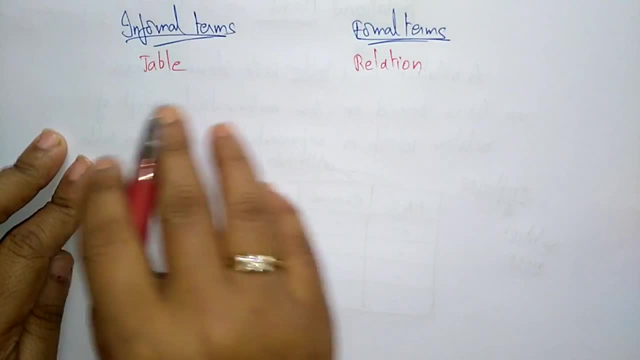 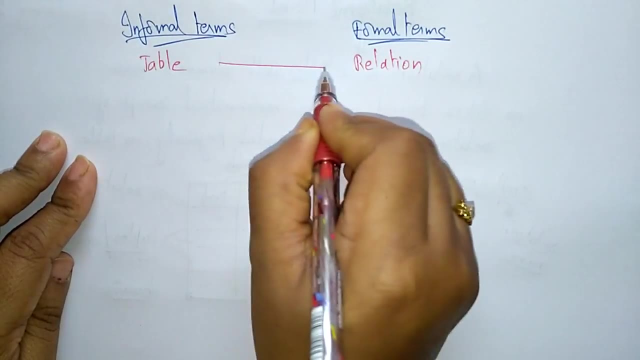 Generally we call it as a table, But in the term of the relational model, Meaning in the term In the name of the table, In the name of the DBMS, The table. The another name for the table is relation. Next. 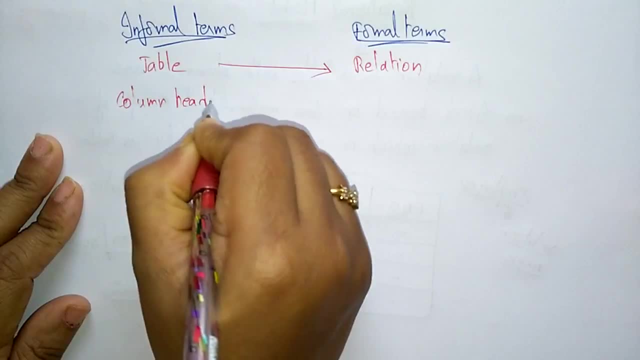 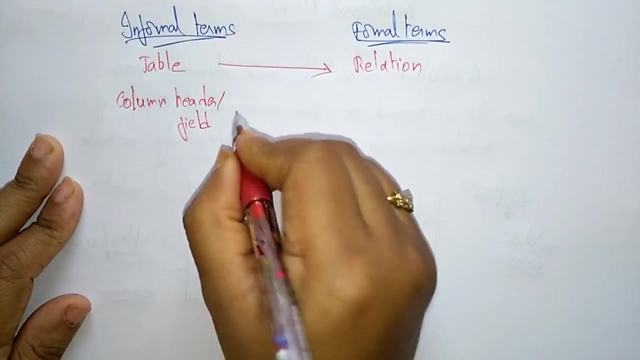 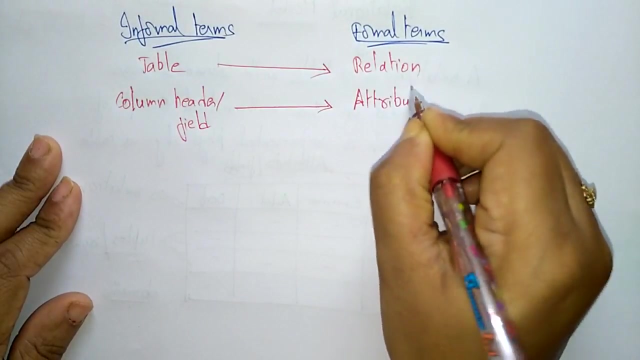 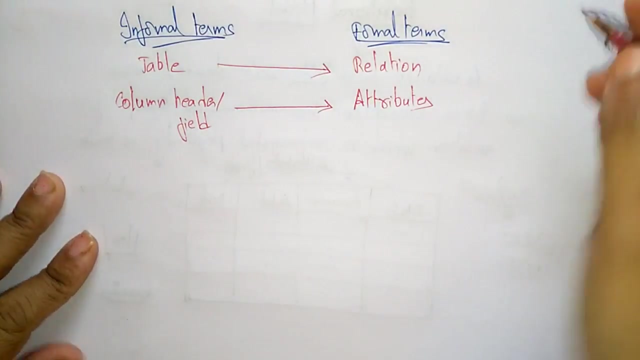 Column header. So column header is also called as a field. Okay, You take it as a field. The formal term for the column header is attributes. So in the term of the database management system, The In a table you are having the column headers means these are the headers. 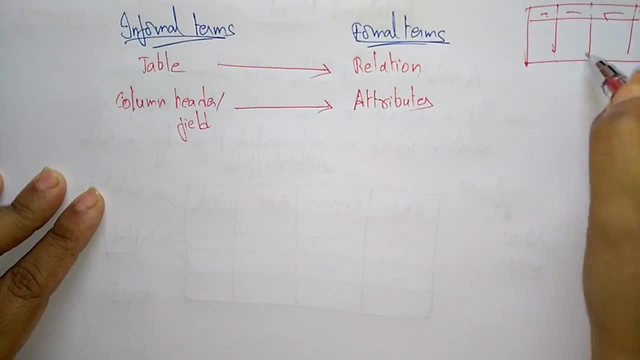 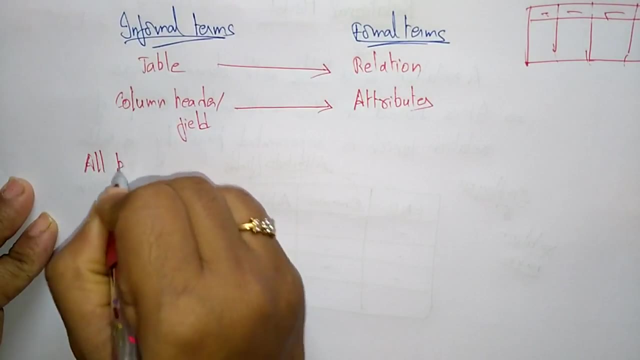 These are the headers of the table. So these headers, you call it as attributes, Next coming to All possible Column values. So I'm not talking about the header, I'm talking about the column values. So all the values In this. 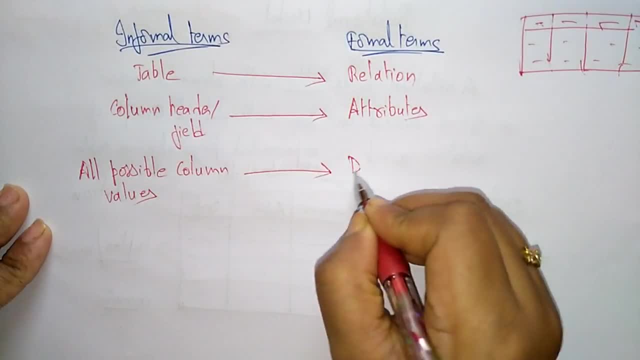 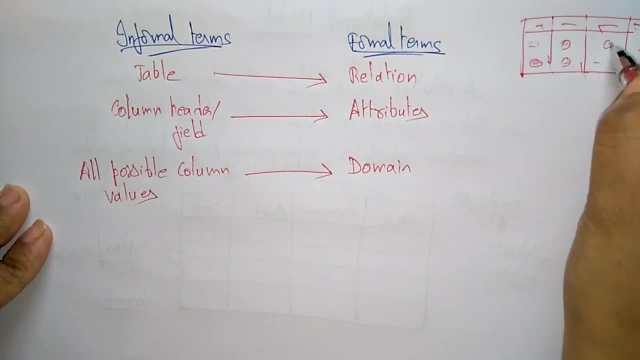 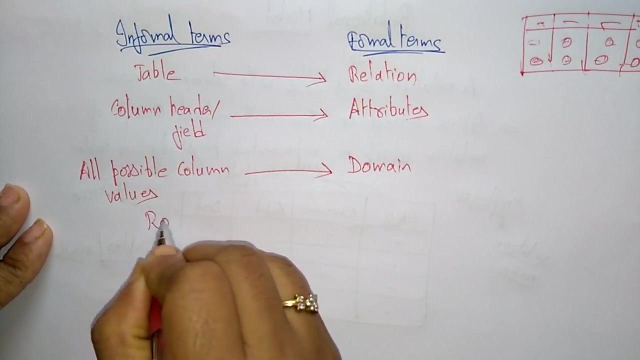 Columns, you call it as domain. So all possible column values, Whatever the values that are present in a table, Those values you call it as a domain. Now coming to the row, So what is the each row In a table, you call: 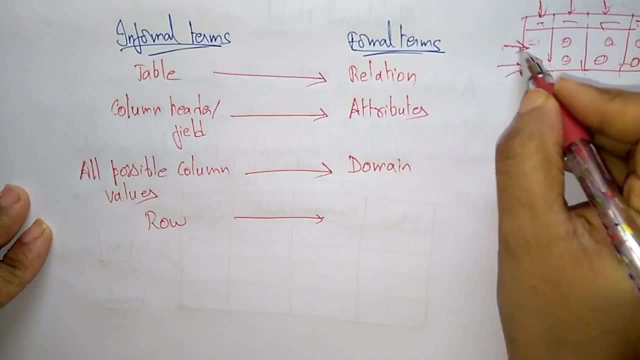 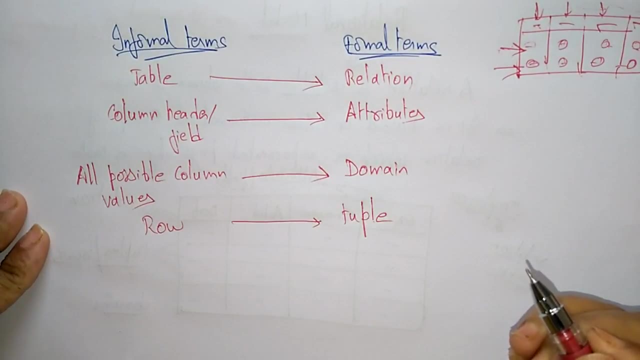 So fields are the attributes. And coming to the rows, Each row in a table, you call it as A tuple, Tuple, Tuple, Okay. Next, coming to what is then another name for the table definition, So table definition. The formal term for this table definition is schema of relation. 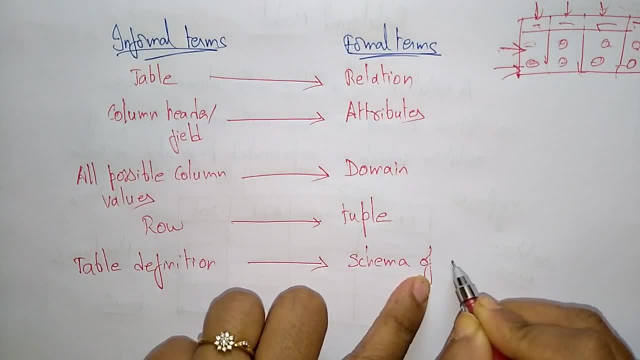 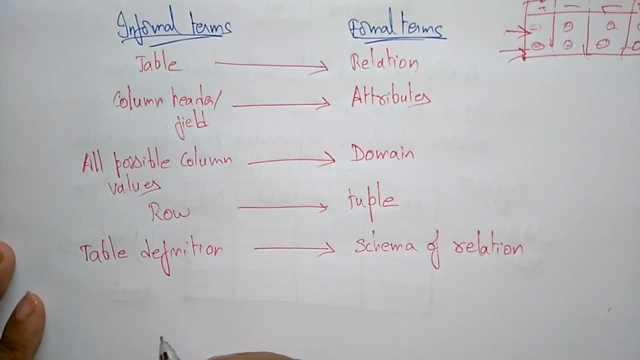 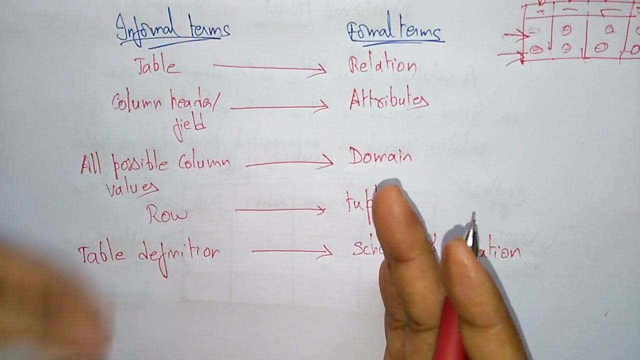 Schema is nothing but a definition. Definition of a table Means the definition of a relation, Schema of relation. Okay, So these are all the informal terms. So informal terms, we already means the general terms that are used while you're talking regarding the tables. 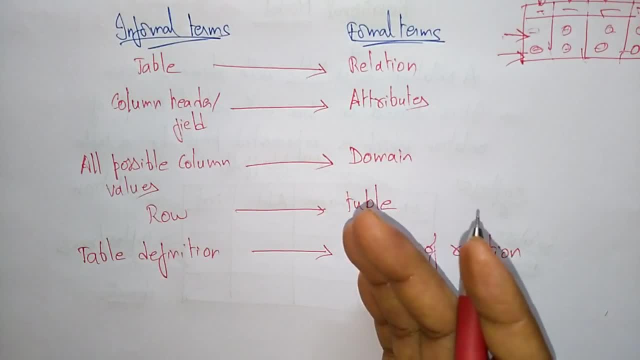 Means. we just if you take the table, we take it, we call it as a table and that fields that are present, you call it as a headers and the way you call it as a values and this completely you call it as a definition, But whereas you coming to the formal terms, 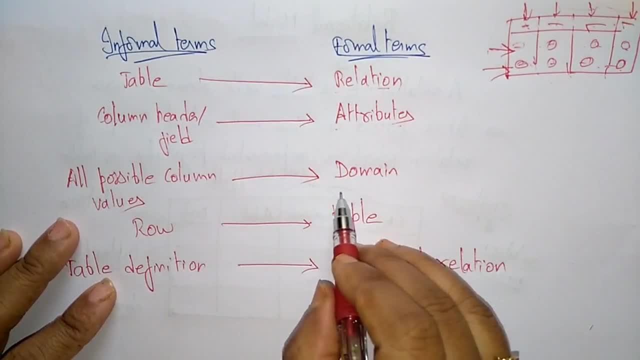 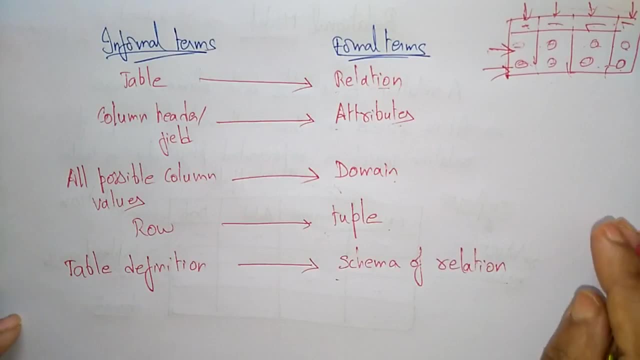 A table is a relation, A field is an attribute, The values- you call it as a domain And the rows, you call it as a Tuple. and the definition of a table is a schema of relation. So these are the formal and informal terms. 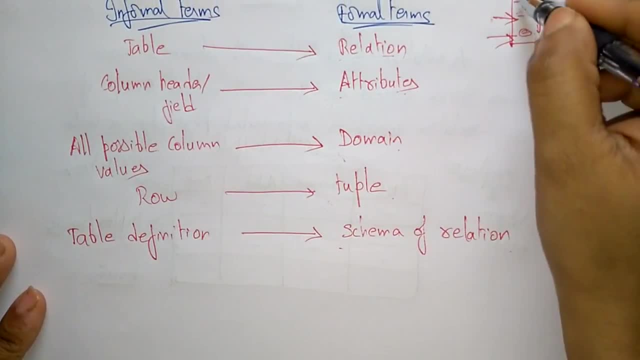 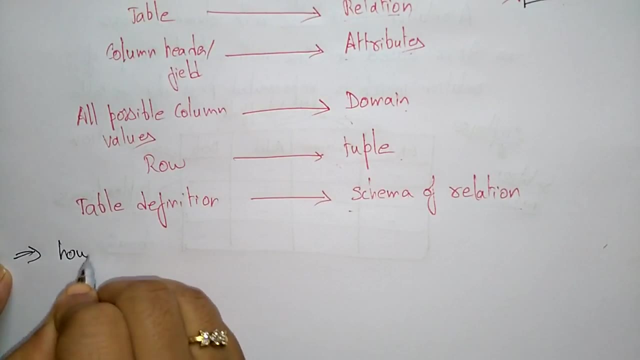 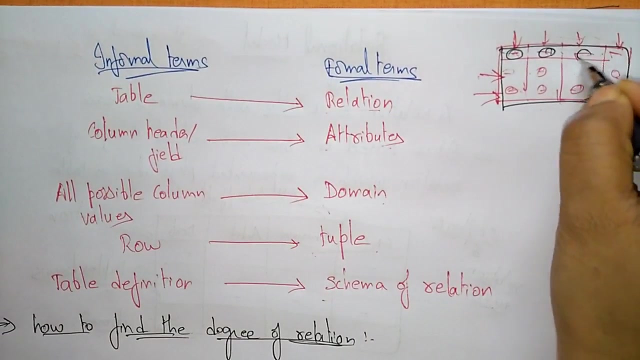 Now let us see how to find the degree of a relation. Suppose, if you want to find the degree of this relation, this table, How will find How to find The degree of Relation? So The only the pointer To find out the degree of relation is number of attributes in a relations means based on the number of the fields, number of the columns that are present in the table that you call it as a degree of relation. 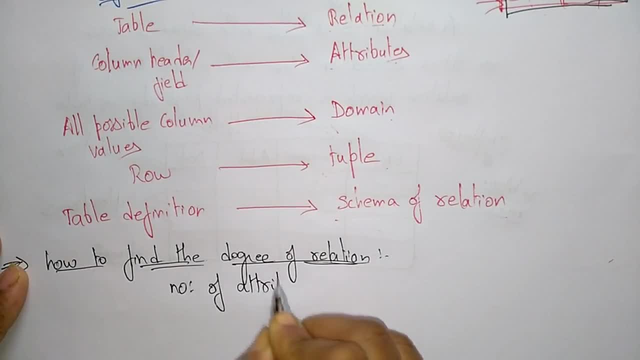 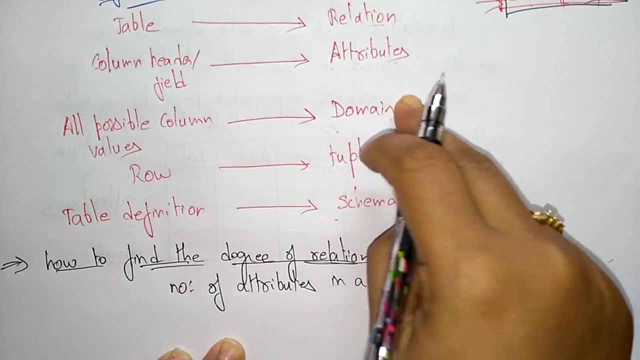 So number of Attributes, Or the fields that are present in a table That is in a relational, So number of attributes in it. and here I'm using the formal terms. So I already said what is an informal term for that: formal terms. 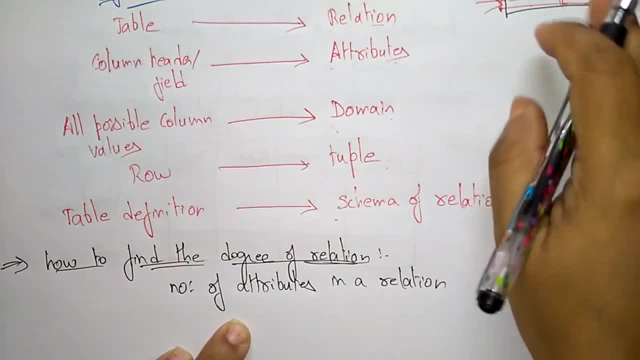 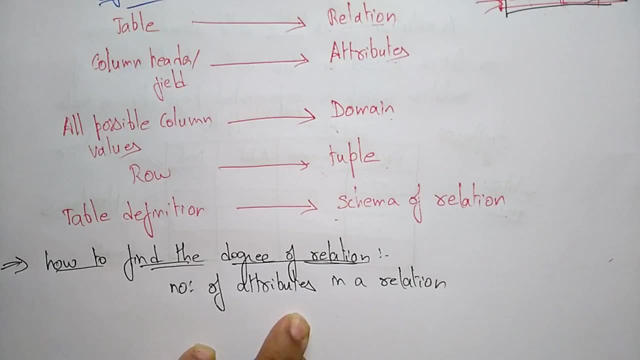 So don't be confused: attributes are nothing but the column, headers or the fields and the relation. then the name for relation is a table. So instead of table I'm just writing a relation. So number of attributes in a relation is called degree, Degree of relation. 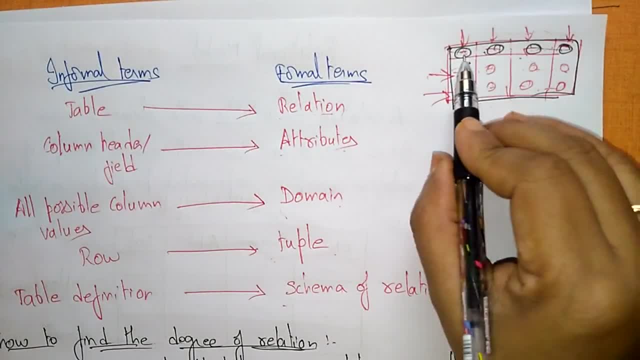 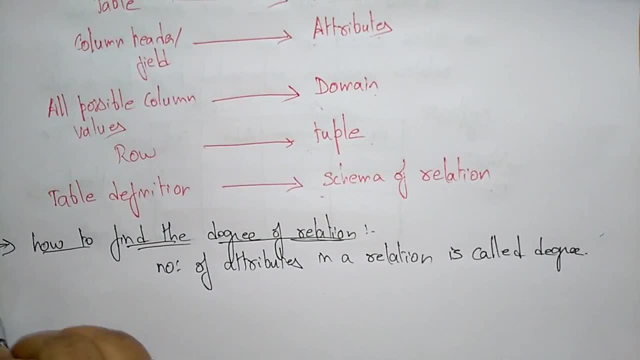 So here, what is the degree of this table for? Because four columns, Four attributes, Attributes are there. So that's why the degree of this table is the four. Next, How to find cardinality of relation. So in this video I'm just giving the more the basic terms that are used in a table. 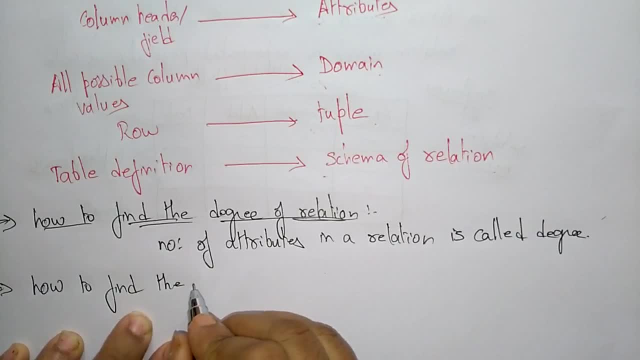 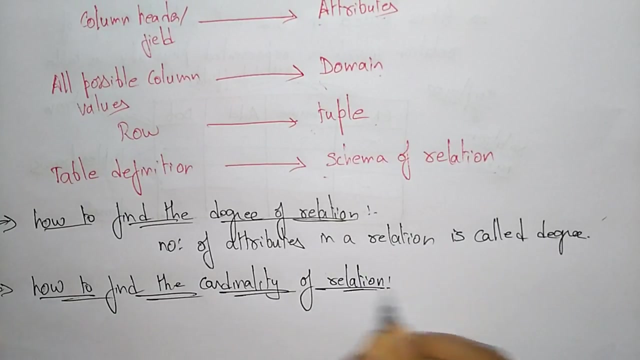 While you're discussing about the relational model, Find how to find the Cardinality Of relation. So how to find the cardinality? So here the degree is based upon number of attributes, whereas cardinality is number of Couples: Number of couples contained in a relation. 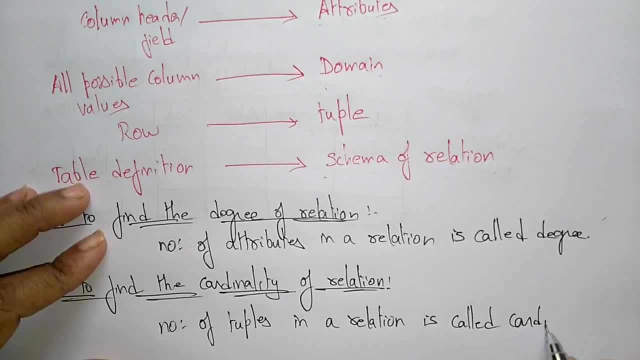 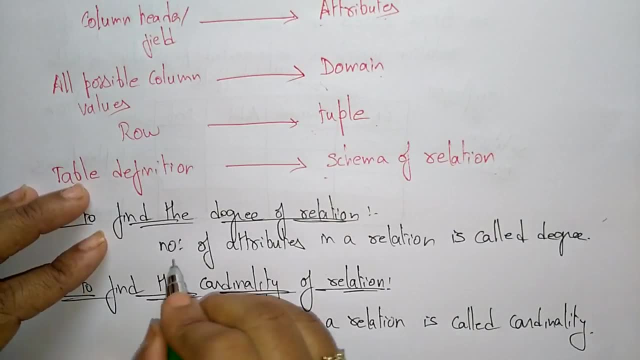 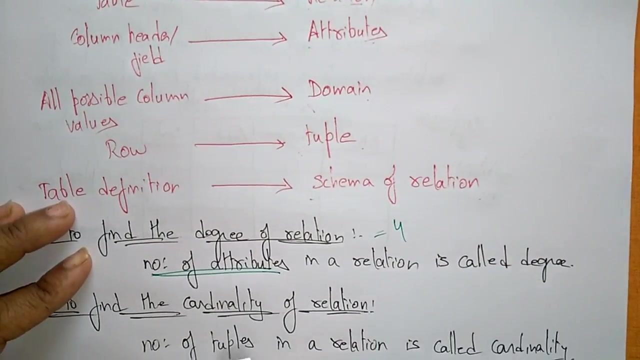 Is called cardinality. So the only difference between here is to find the degree of relation. You need to know the number of attributes present in a relation. So here you're having the four attributes. so the degree is here is a four. Find the cardinality of relation means number of couples in a relation. 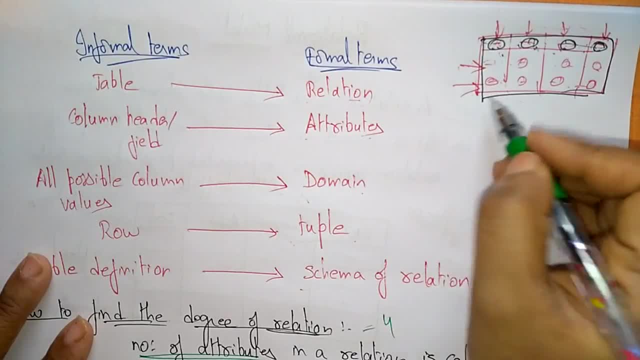 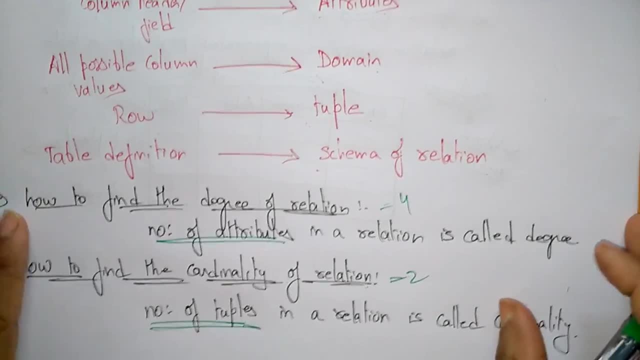 Couples means rows. So how many couples are there Here? only two. Two rows are there in this table. So number of couples in a relation: you call it as a cardinality. So these are the terms that are used in the relational model. 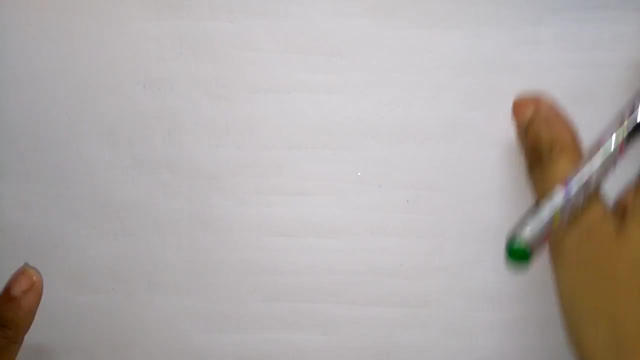 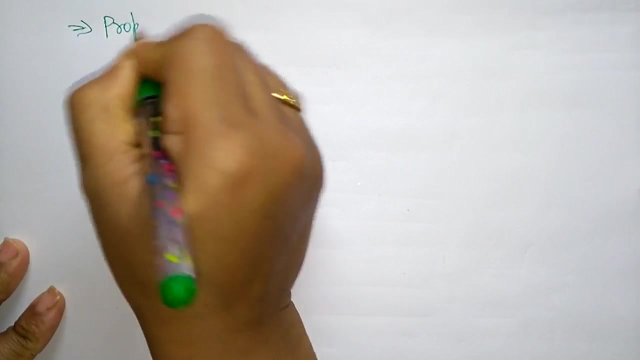 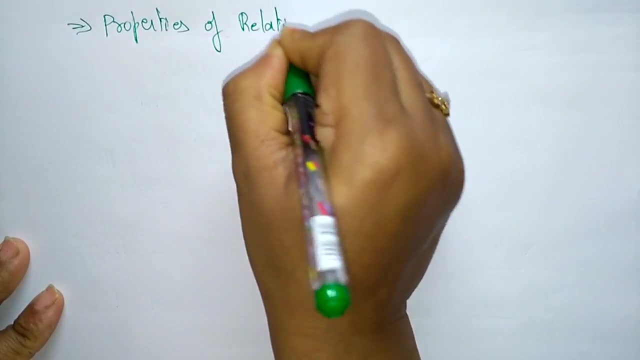 Now let us see some properties, Properties of relation. so before you're going to know about the complete relational model, you have to know the properties. what are the properties that are involved while you're creating it? tables means the relations, properties of Relation. So the first property is: 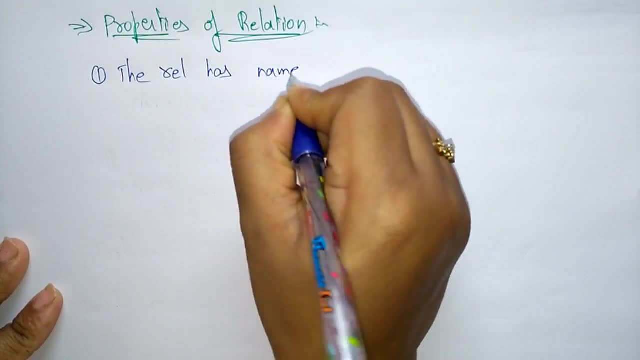 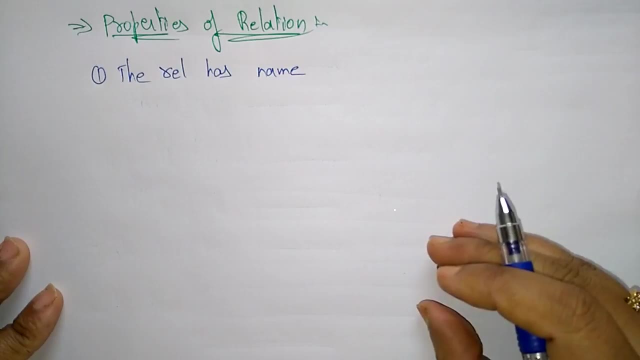 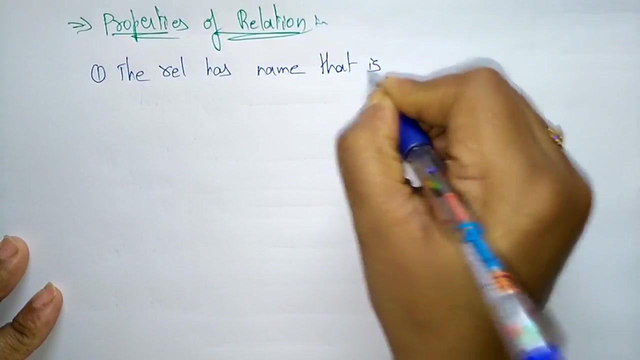 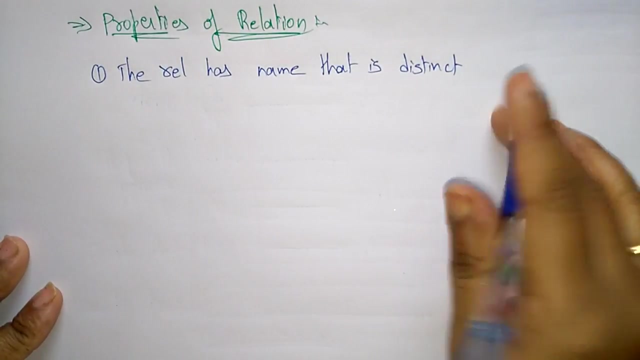 The relation has Name. So every table Should be Declared with a name. means without name you can't identify the table. so the relation- the table has name that is Distinct means each table has a unique name. means different names. So relation has a name that is distinct from. 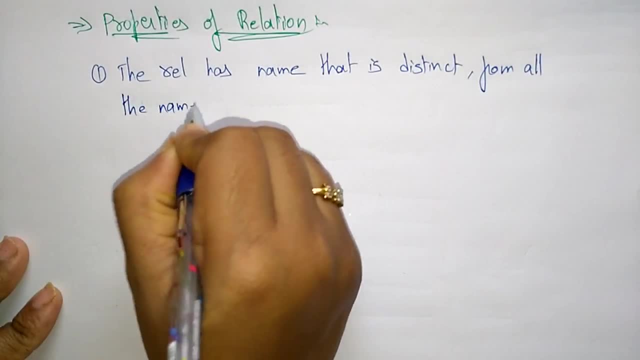 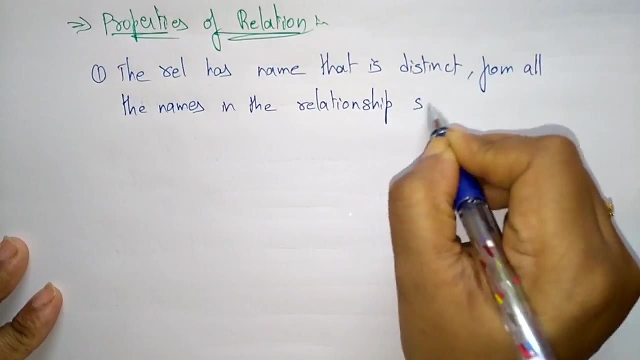 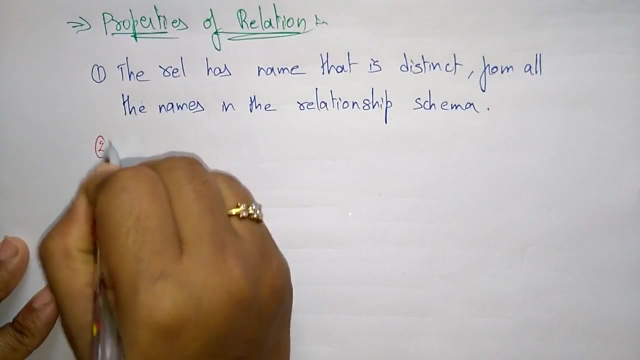 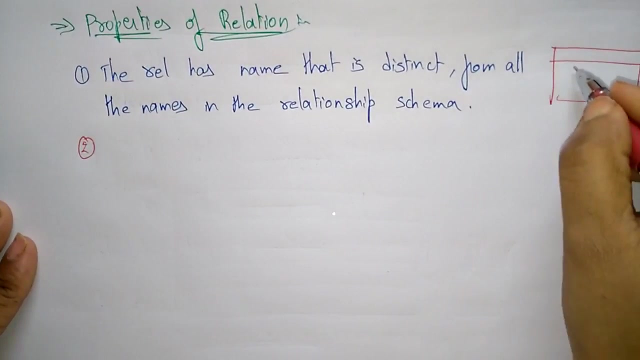 All the names In the relational Relationship schema Means in the complete definitions of a table. you have to declare each table with a different name. Next point: each cell of the relation means the cell you call it, as this is a table. so in the table you are having the, this is the attributes, and here these are the. 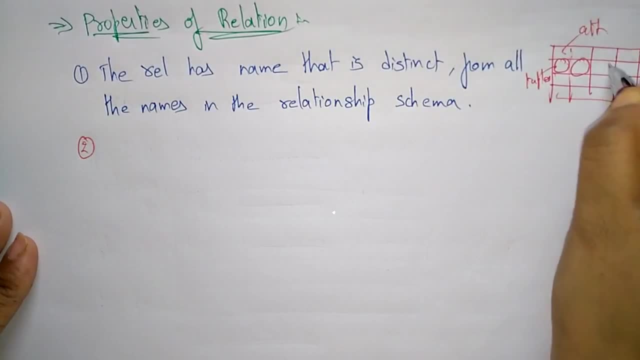 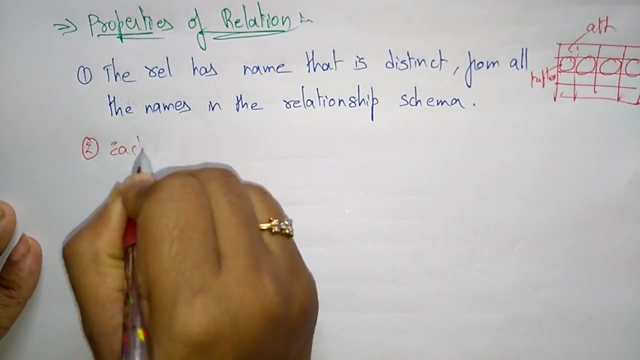 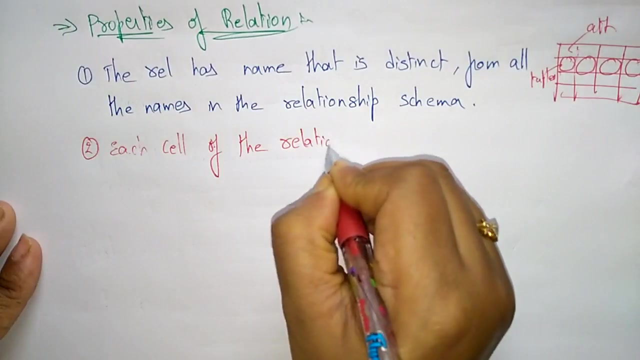 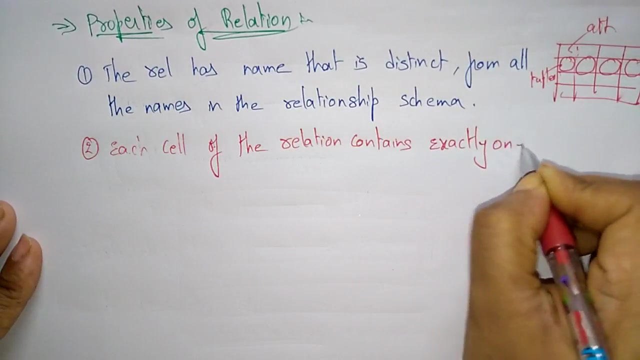 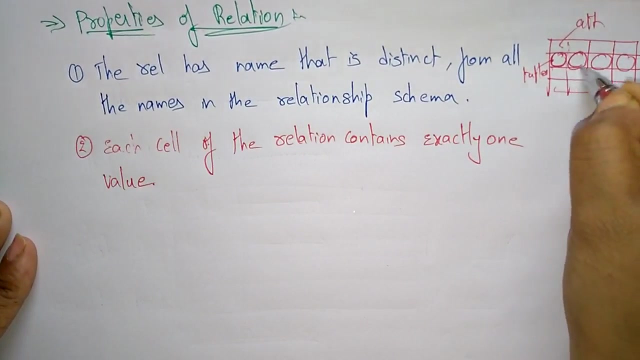 Couples. so here this you call it as a cell. each. These are the attributes. Each cell Of the relation Contains Exactly one value. So, while you're creating the relation, while you're creating the tables, you have to be careful That each cell, whatever the values that are present in each cell, 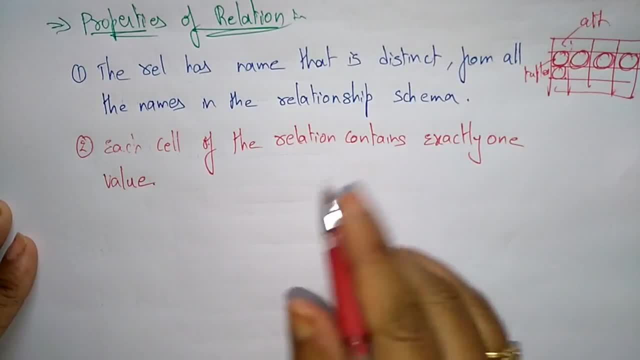 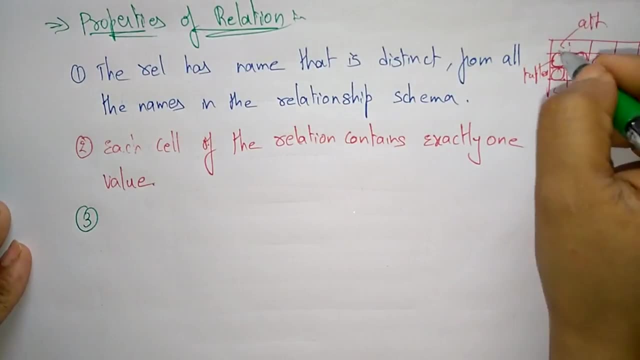 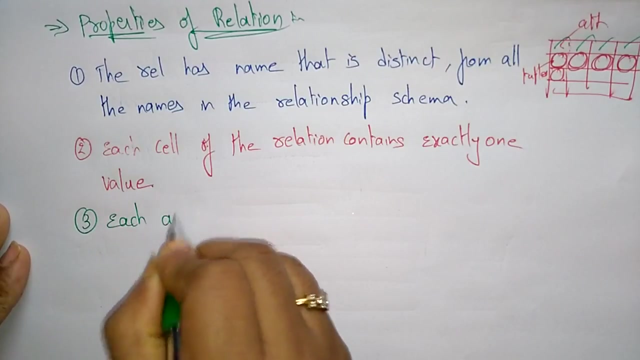 Should contain only one value, exactly one value. and coming to the third point, here, each attribute had distinct names. so if you take the column name, the column name should be distinct. each attribute has distinct, distinct means, different, distinct names. so here, suppose, if you write the name again you are not supposed to. 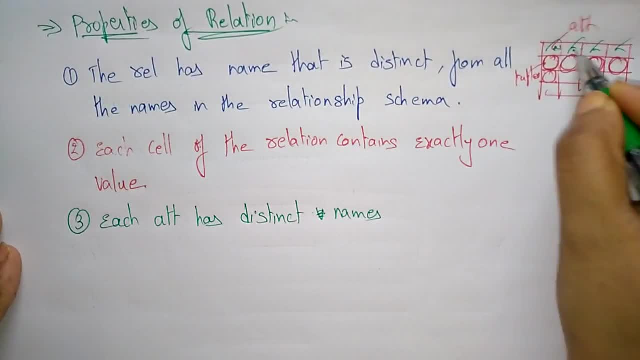 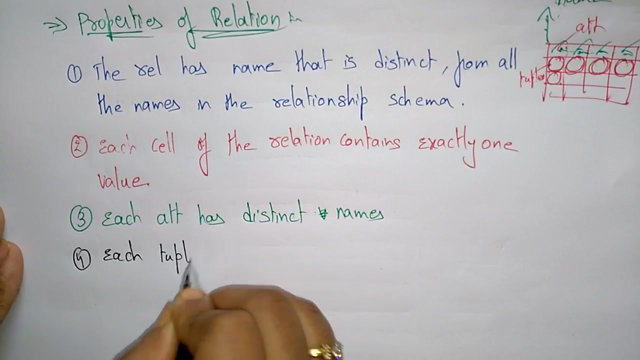 write the name here, so these will be different. each attribute name should be different. the first point is: each relation has a name, should be there relational name and each cell should contain only exactly one value and each attribute has distinct names. fourth point: each tuple means row. each tuple. 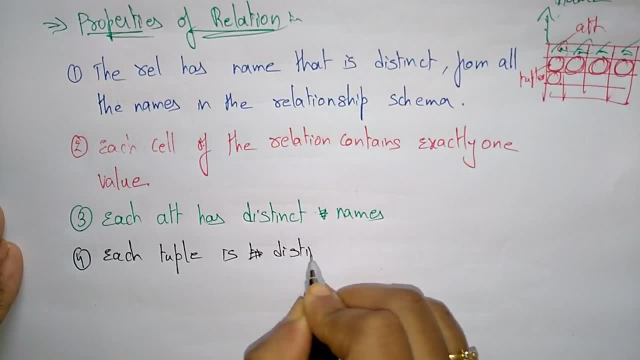 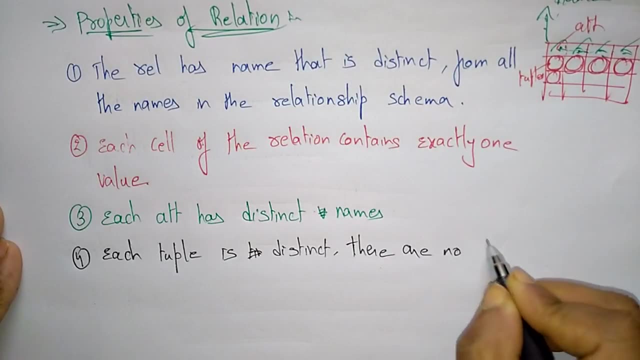 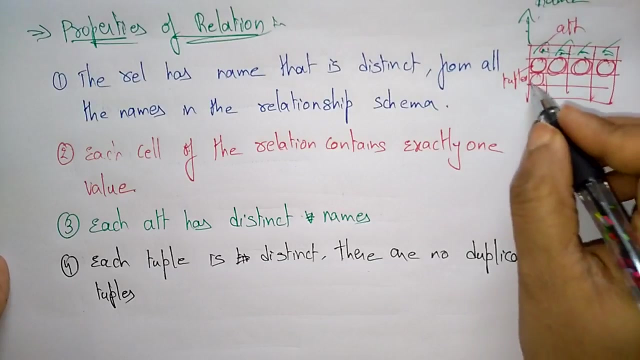 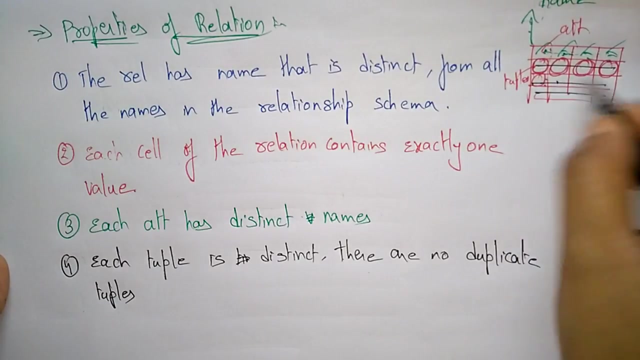 is distinct. okay, okay, so distinct. there are no duplicate tuples. there are no duplicate tuples means the complete tuple. means the complete row should not be duplicate. maybe columns may, two columns may be unique, but complete row should not be duplicate. means the same value. suppose a name: one, two, three, this is in one row. 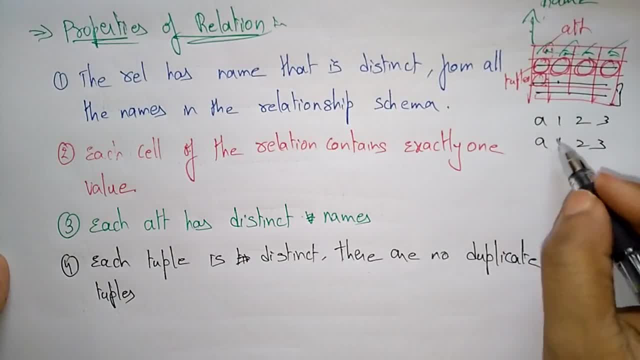 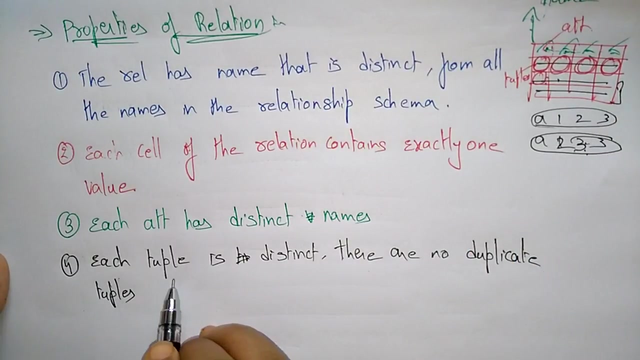 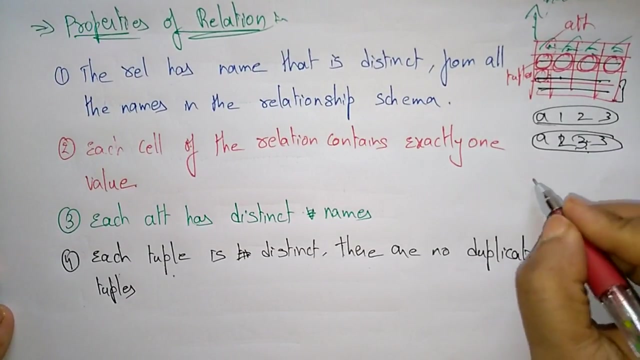 again. a123 should not be present, okay, so the values maybe change. okay, but the same values, the same tuples should not be there in a table. that should be, uh, taking care while you are creating the tables. each tuple means each row is distinct. there are no duplicate tuples. means a111- a111 is not.